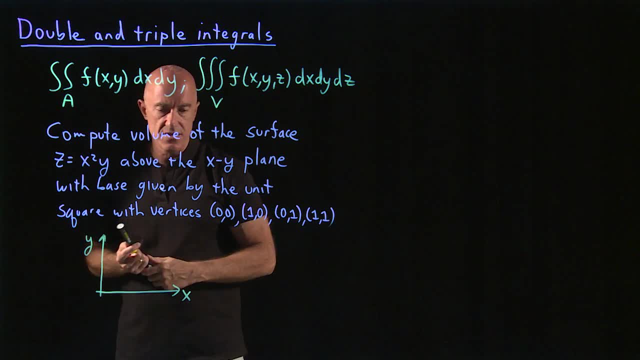 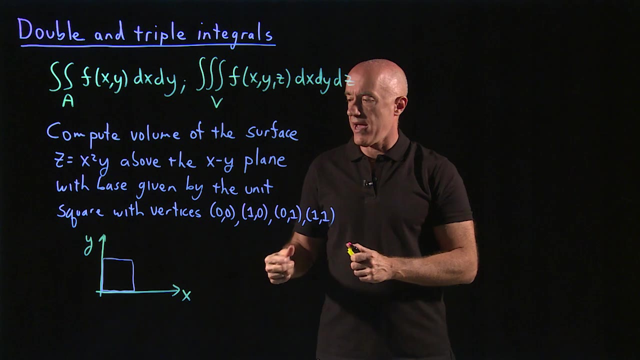 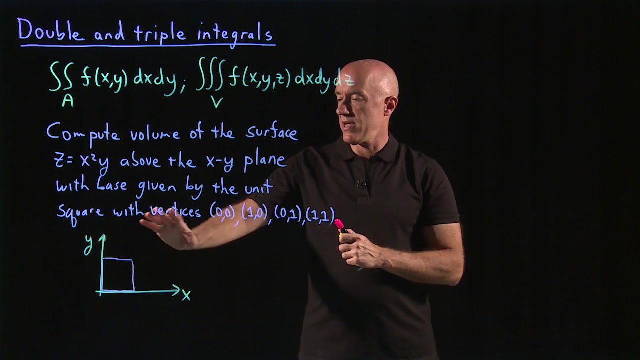 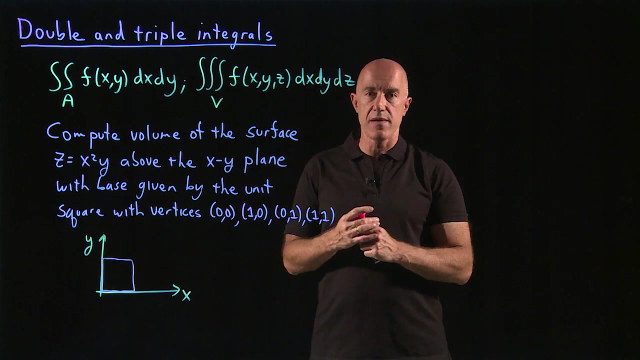 So the base is just a square, So it's just this square, And the surface is z equals x squared y. So we want to find essentially what is a volume between the surface x squared y and this Square in the x- y plane. Okay, So a double integral, then, can be interpreted as a volume. 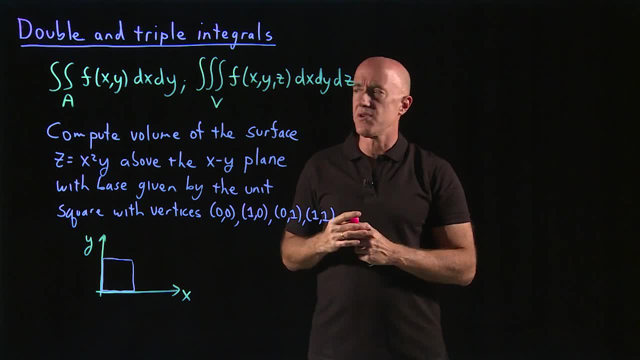 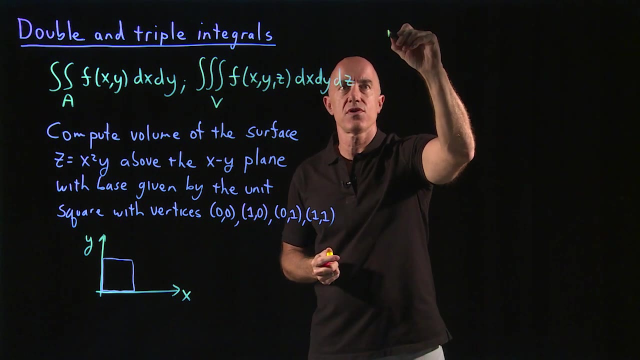 just like a single integral is the area under the curve, The double integral is the volume under this function, f of x, y. Okay, So how do we set this up? So I'm going to show you two ways of doing this. So in 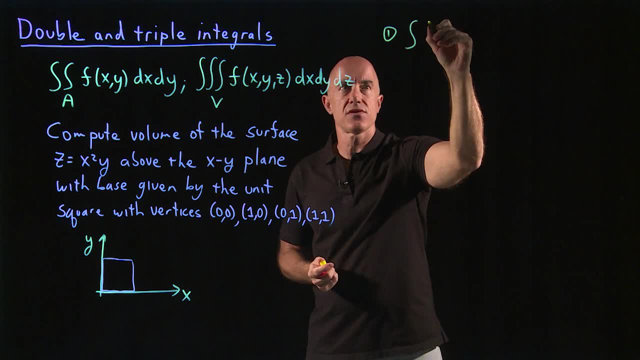 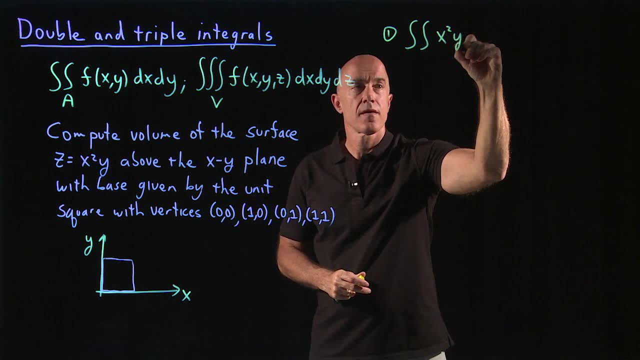 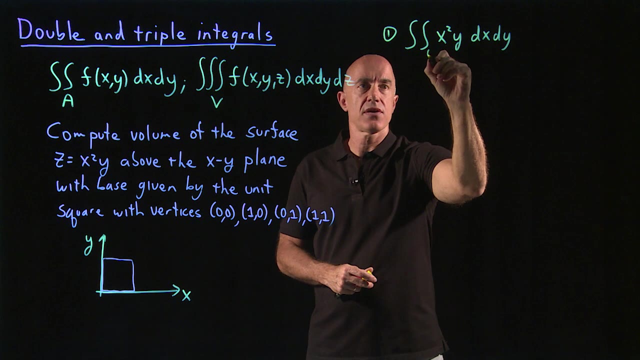 the first way we're going to do a double integral. So we're going to do a double integral of the function which is x squared y, And we can integrate dx, dy, x goes from 0 to 1.. y goes from 0 to 1.. So when you write this: 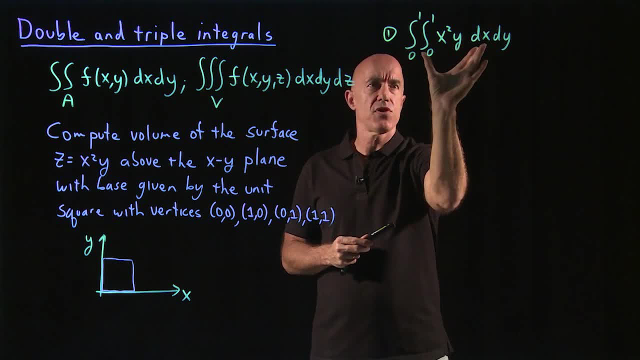 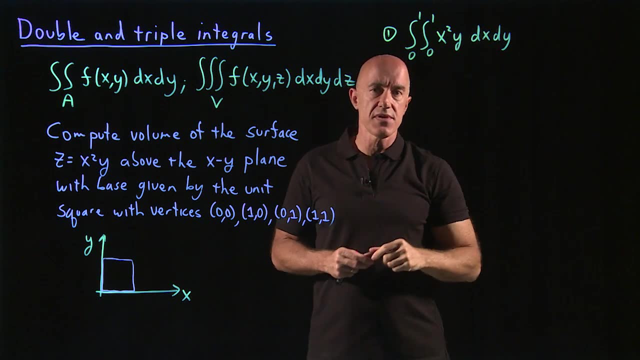 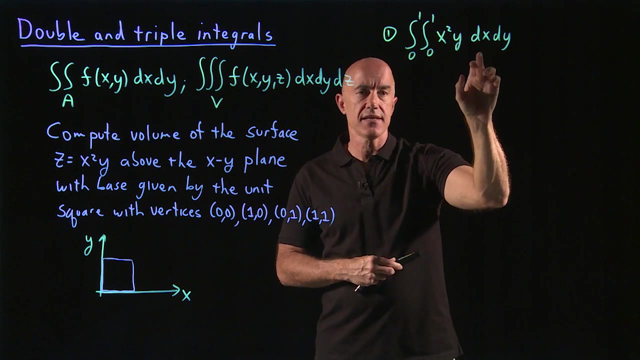 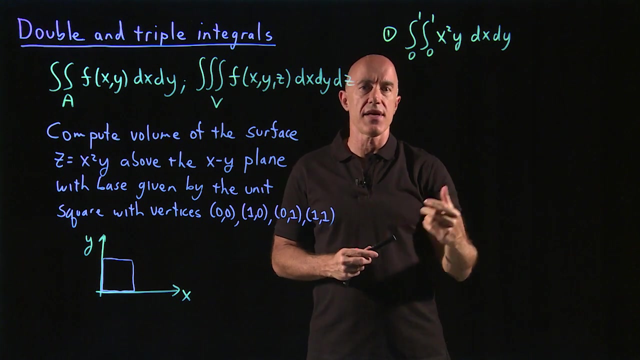 integral. the meaning is you do the first integral, dx, first. So the dx, the first integral, friends, which is the infinite sets small element, dx means that the first integral corresponds to integrating x, dx And the second integral corresponds to integrating dy. And in a case like this, you just do them. 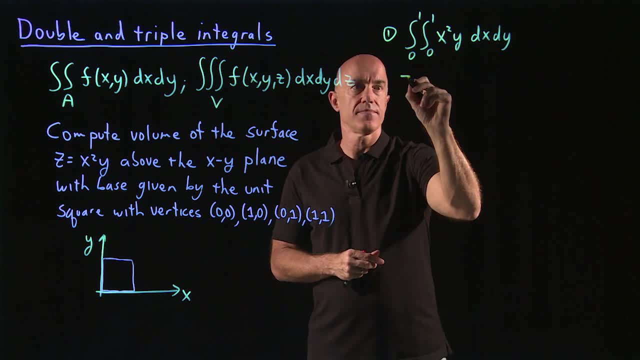 sequentially. So first you integrate over x, keeping y fixed. So if we integrate this over x, we still have 0 to 1. And then we integrate x squared Yoon from 1. All we got is dx, So the firstyingabor angles. and then we continue Here. what we an do can be that is this: It's: going to be constant respuestafit, So this will be string Yin. we have all theBean equations, Thisği Barangdenha equation, So we do it across ל and we're going to integrate realün flareliureum the position plane A and X boundaries twice, both strings in right square, once two. Look here. 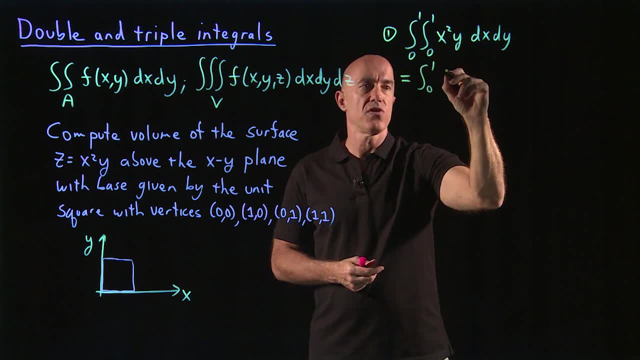 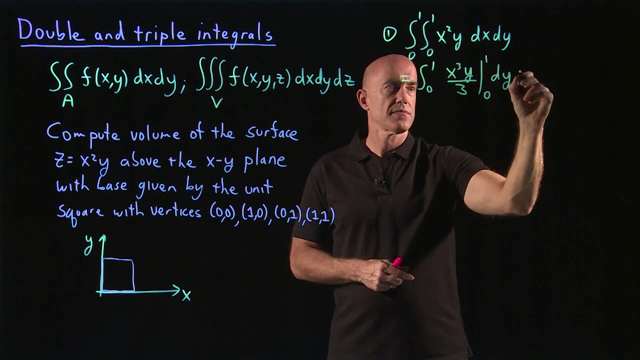 squared, keeping y fixed will be x cubed over 3, so x cubed y over 3, and that will be as x goes from 0 to 1, and then we'll have a dy integral left. So this is the value. 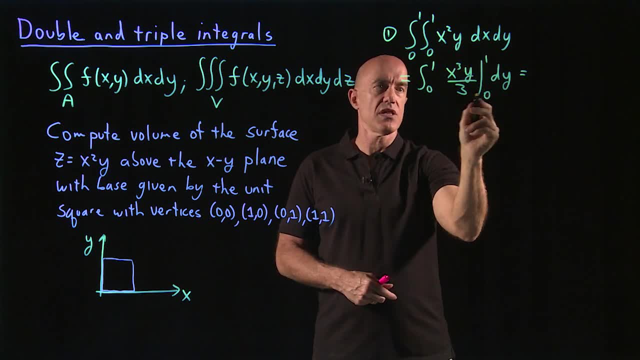 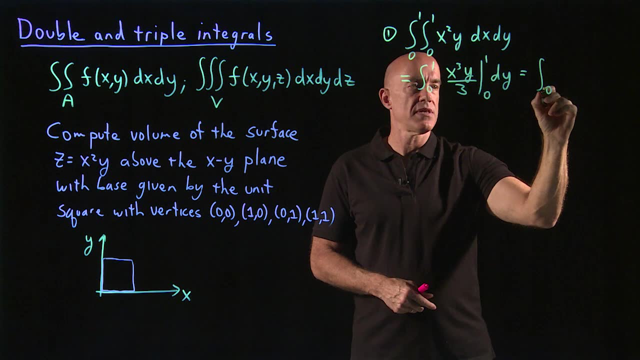 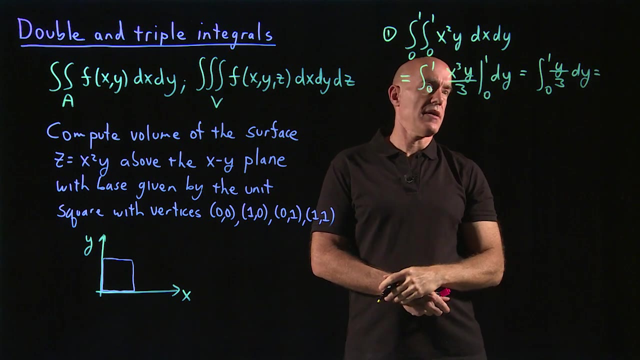 of x. now we integrated x, so the lower limit will be 0, the upper limit will give us a y over 3, so this will be an integral from 0 to 1, y over 3, dy. then this is y squared. 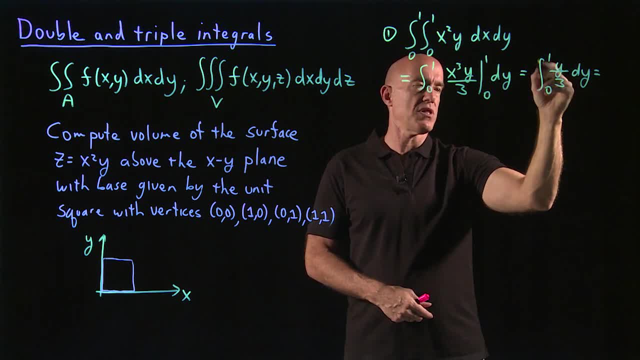 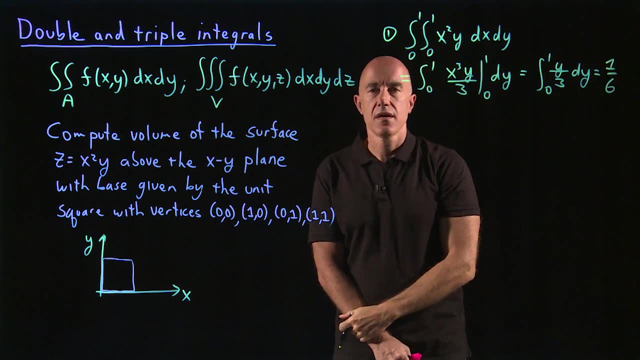 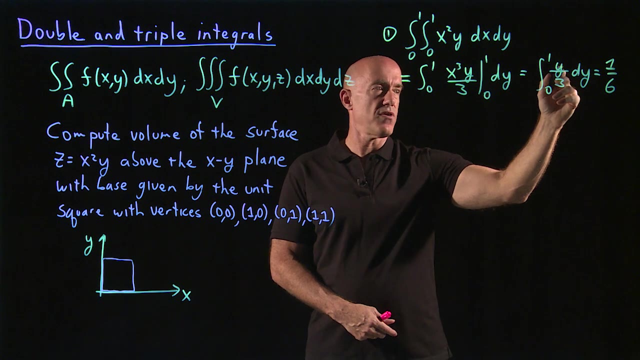 over 2, and we plug in the upper limit 1, which will be 1, 6.. I hope you can do that in your head, so I'm going to try to save some space here. So squared over 2 will give us 1, 6.. 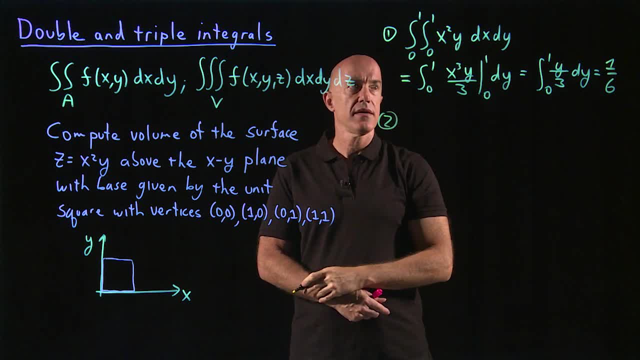 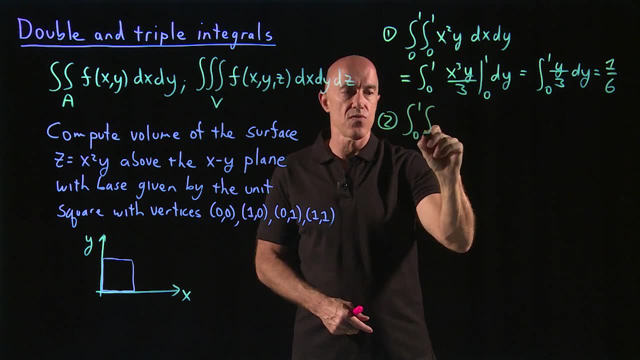 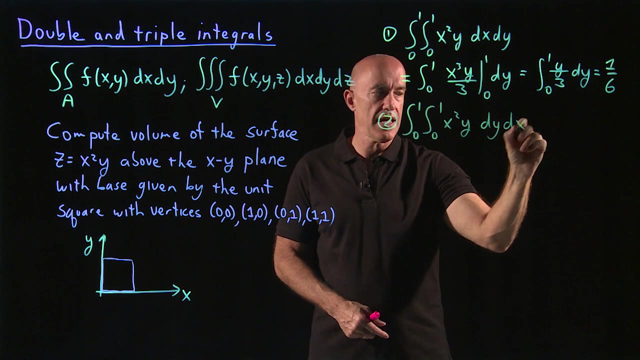 So that's the first way. The second way, instead of integrating x first, we could integrate y first, So we could have the integral from 0 to 1,, 0 to 1, x squared y. But now we integrate dy dx. okay. 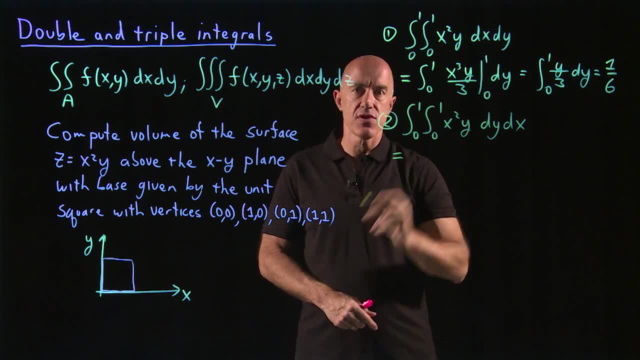 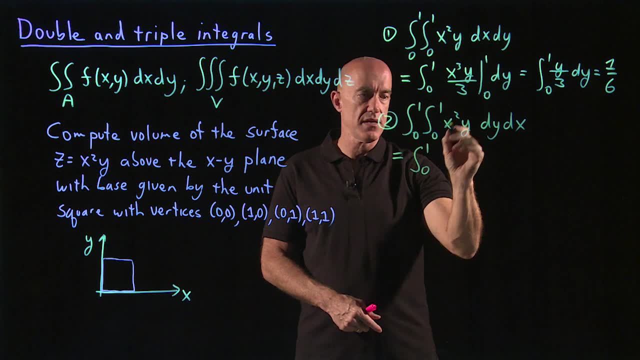 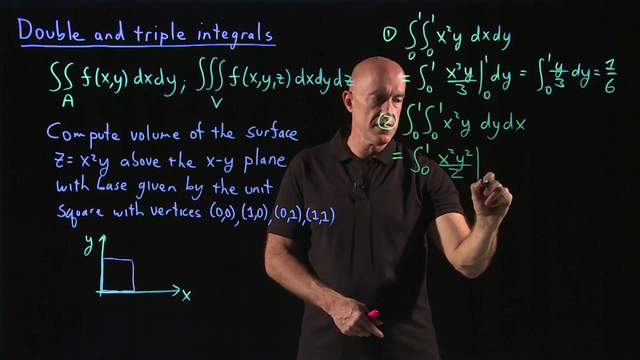 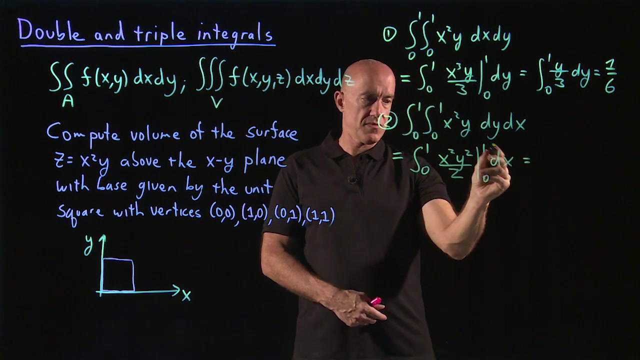 What would this be? So now we integrate y first, keeping x fixed, so it becomes y squared over 2.. So the outer integral is 0 to 1, and then we have an x squared, y squared, divided by 2, between the limits 0 and 1 and dx. 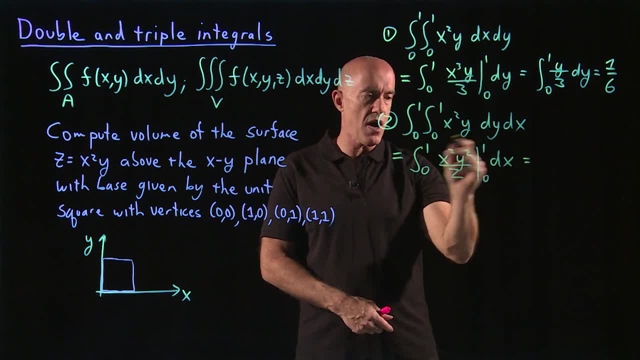 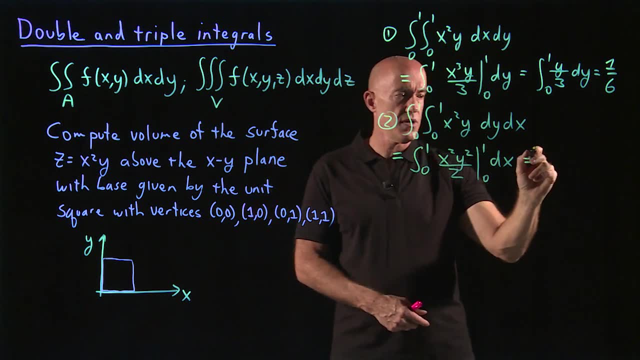 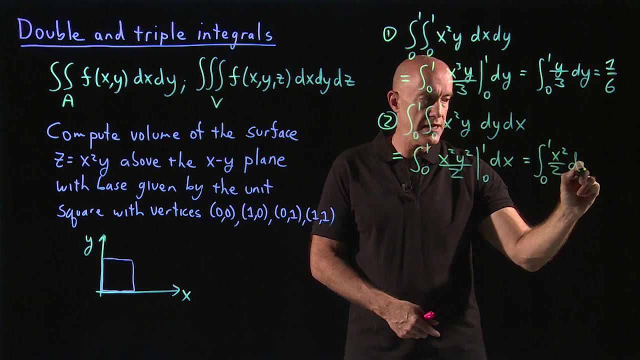 So now this limit here corresponds to the limit of y. The lower limit will be 0.. Okay, So the upper limit will be x squared over 2.. So this is the integral from 0 to 1 of x squared over 2 dx. 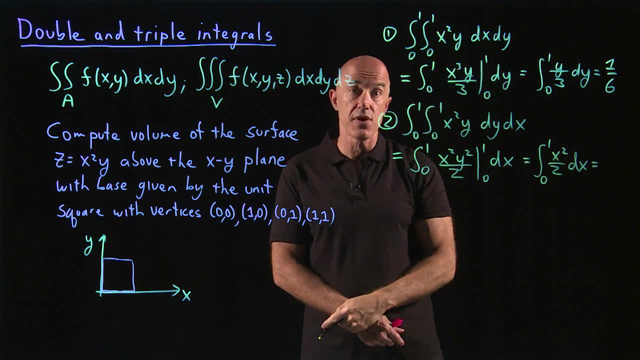 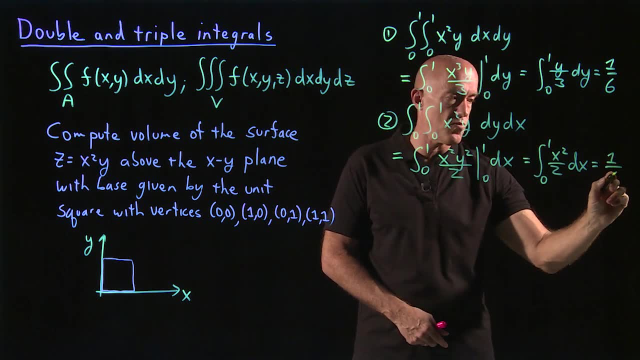 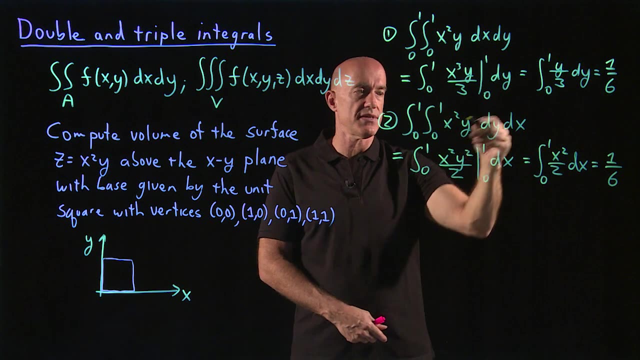 This becomes x cubed over 2 times 3, which is 1,, 6 in the upper limit and 0 in the lower limit. So again we get 1, 6.. Okay, So this first one is: integrate x first. 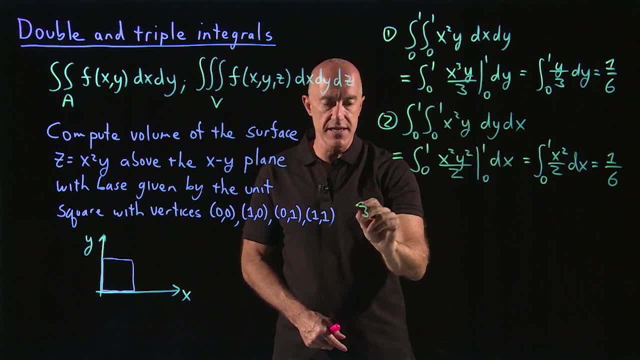 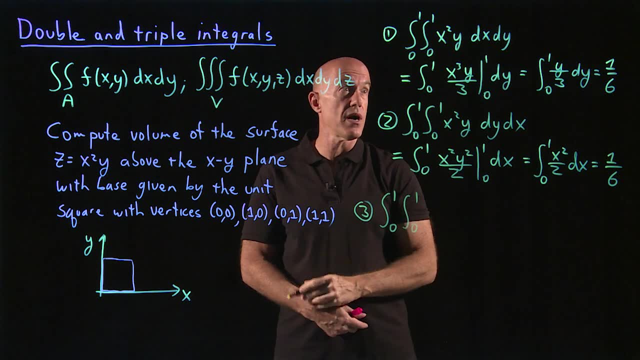 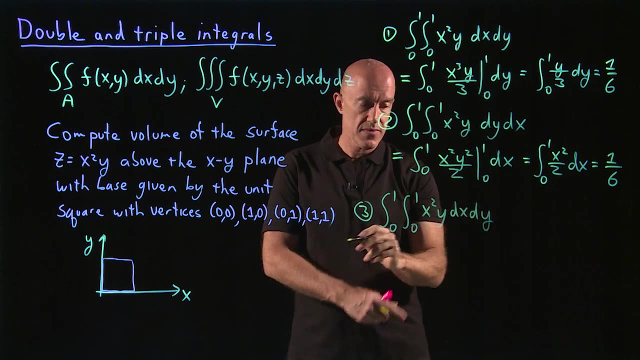 The second is integrate y. In this particular problem we can actually shortcut this. We have integral from 0 to 1,, 0 to 1, say x squared, y, dx, dy, Because these limits don't depend on x and don't depend on y. 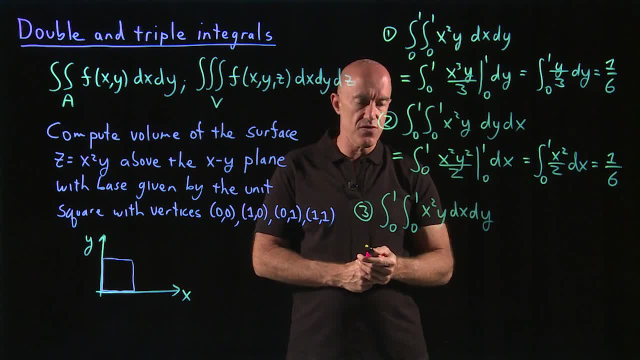 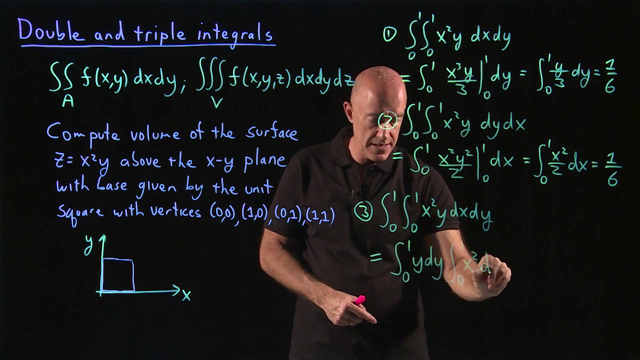 my preferred method for doing this integral would just be to do this. So the x squared dx is the inner one, the y dy is the outer, So you can write this as 0 to 1, y dy times 0 to 1, x squared dx. 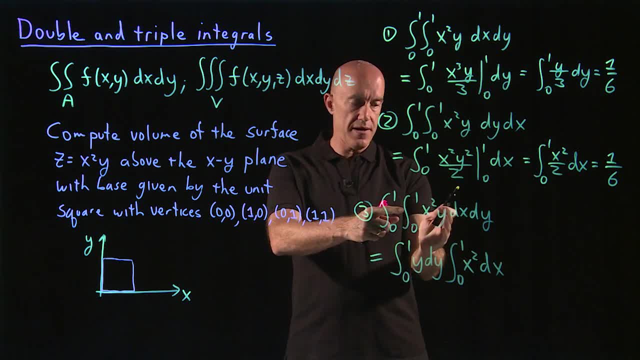 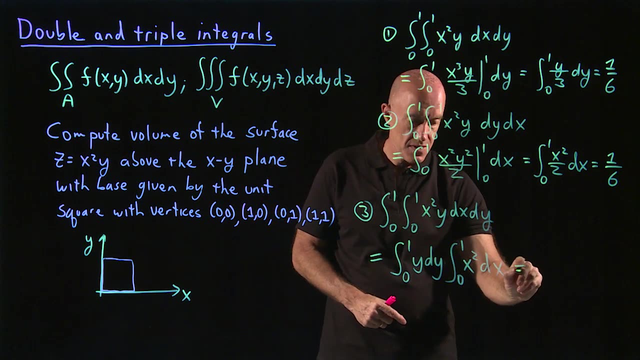 So when the limits don't depend on x and y and x squared y is separable into a function of x times a function of y, Then you can factor the integral. Okay, So this would be my choice. So the integral of y dy is y squared over 2.. 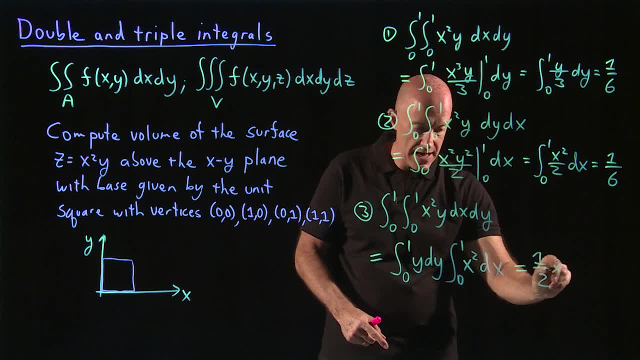 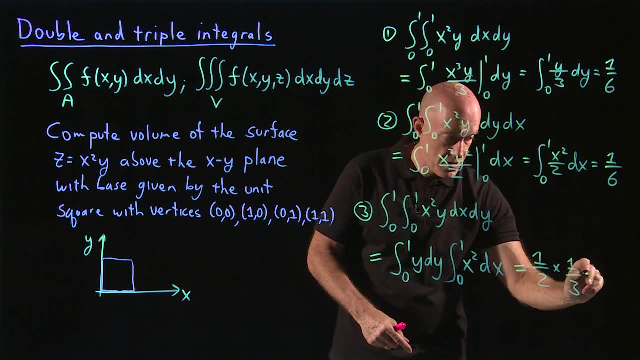 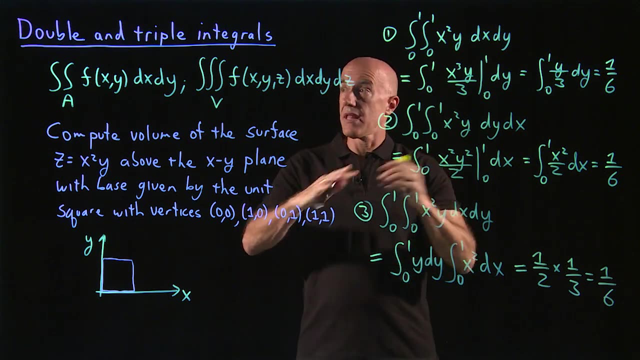 So that would give us a 1 half, And the integral of x squared dx is x cubed over 3.. So that would give us a 1 third, which is a 1, 6 again. Okay. So let me summarize. 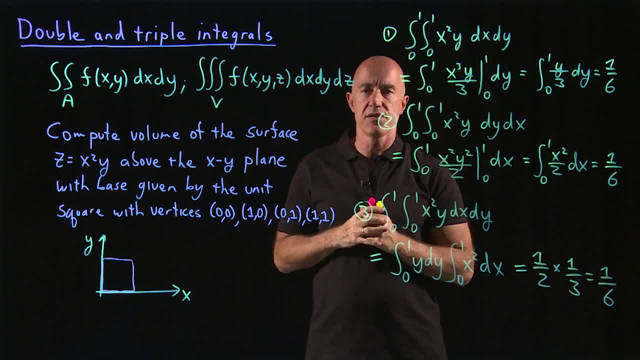 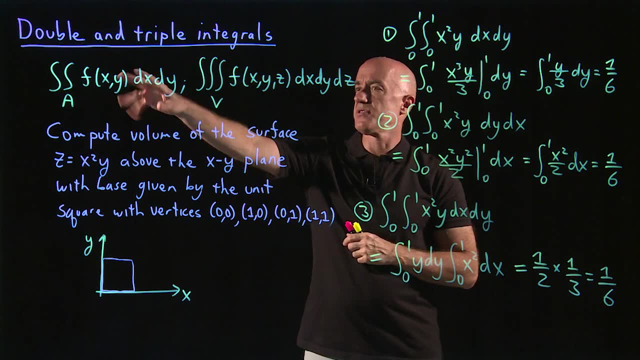 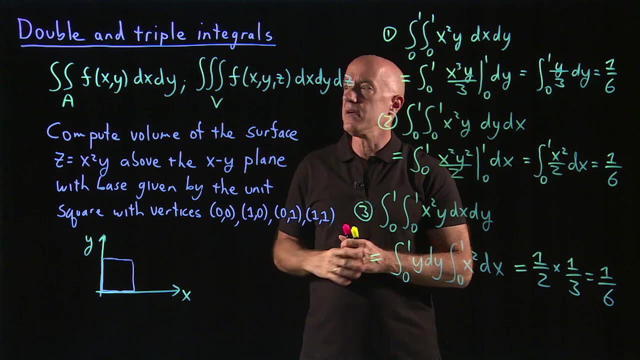 We want to generalize, then single variable integrals to functions of two or three variables. These are called double integrals and triple integrals. A double integral is going to be over some area. A triple integral is going to be over some volume. 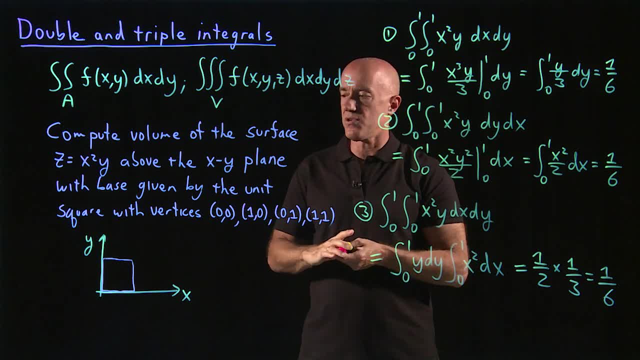 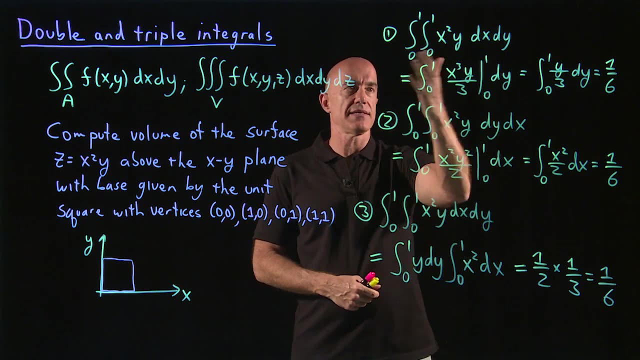 Here I give you what is possibly the simplest type of integral to do. How do you integrate some function here? I call it: z equals x squared y above a square in the xy plane. So I set it up as a double integral of the function dx, dy. 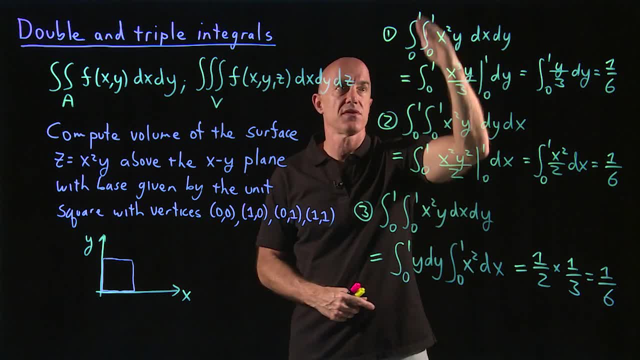 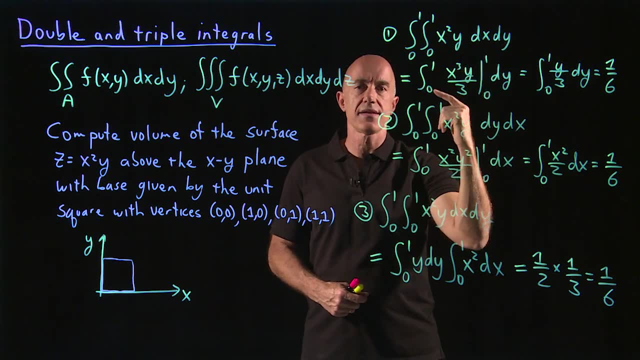 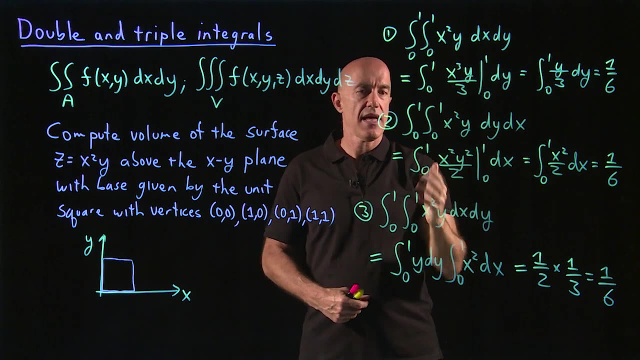 The limits here are corresponding to the limits of x and the limits of y. To do this type of integral, all you do is you do one at a time, So you integrate x first And keeping y fixed, and then you integrate y. 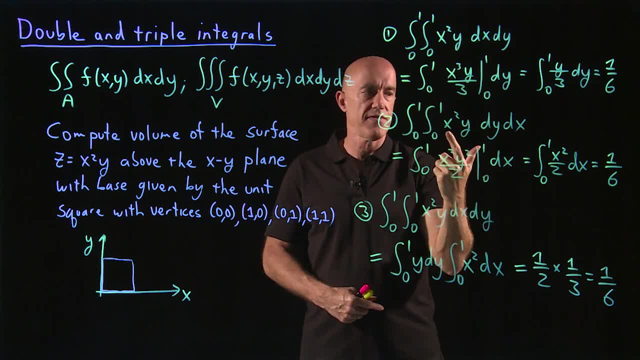 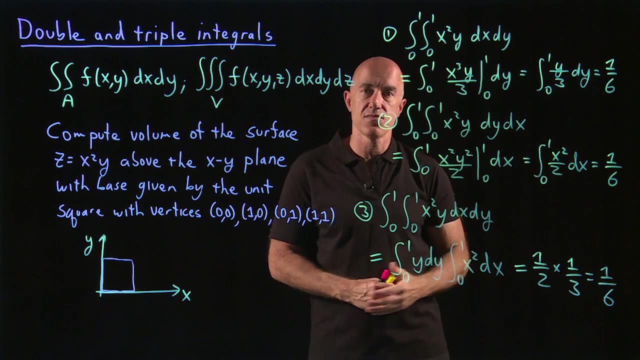 And the second one. I integrated y first, keeping x fixed, And then I integrated x. And then in the third one, I show you that this type of integral is actually factorable, so it factors into two single variable integrals. In all cases we get the answer of 1, 6.. 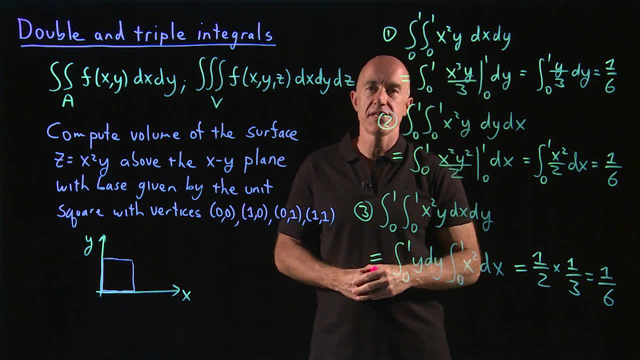 I'm Jeff Chasnoff. thanks for watching and I'll see you in the next video. 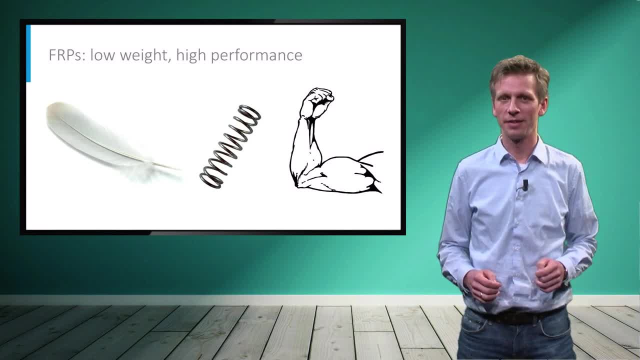 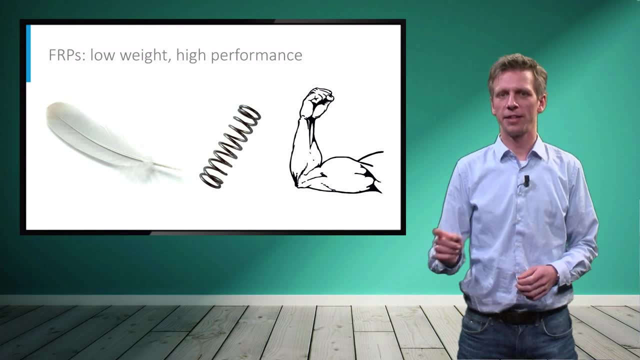 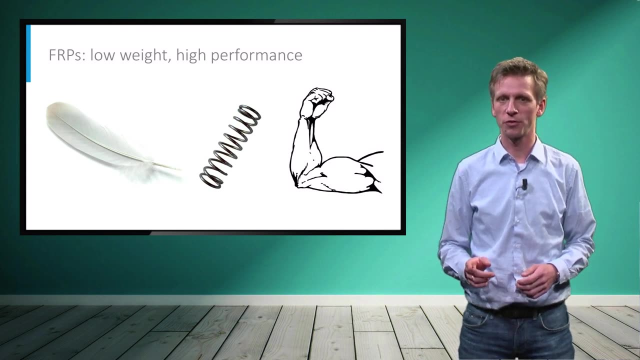 One of the main selling points of FRP composites is that they combine low weight with high strength and relatively high stiffness. It is time to give some numbers to back up this statement. In this video, we are going to compare the mechanical performance of FRPs to that of 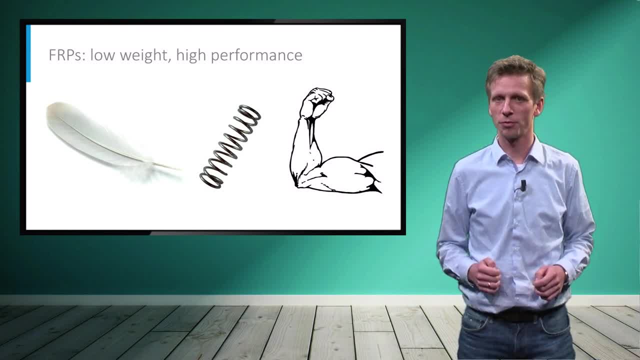 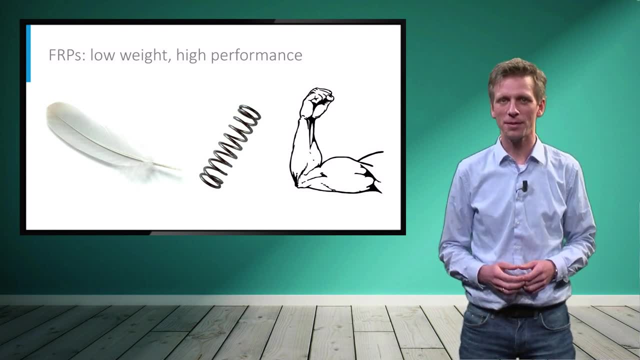 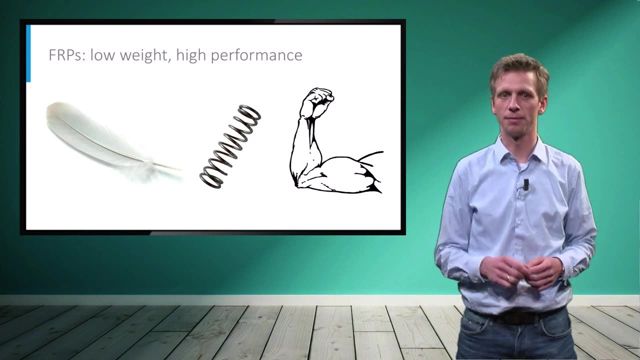 traditional building materials. How is the performance of FRPs in terms of stiffness and strength, And how light is light weight actually? We will compare with concrete and steel, but also include the light weight metal alloys of aluminum and titanium. Let's first consider stiffness. 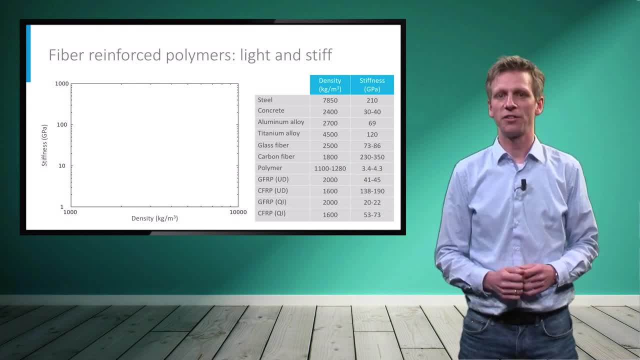 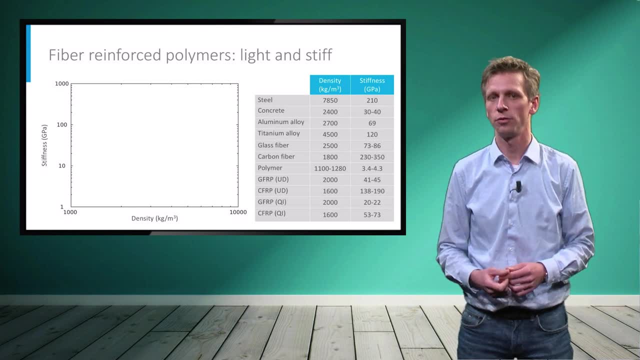 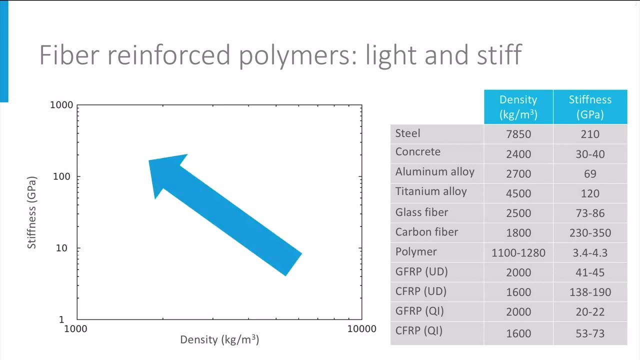 We will plot the stiffness versus density to classify the different materials. The plot is in log-log space so that we can cover different orders of magnitude in the stiffness. Our ideal material is going to be located in the top left corner: Low weight and high stiffness. 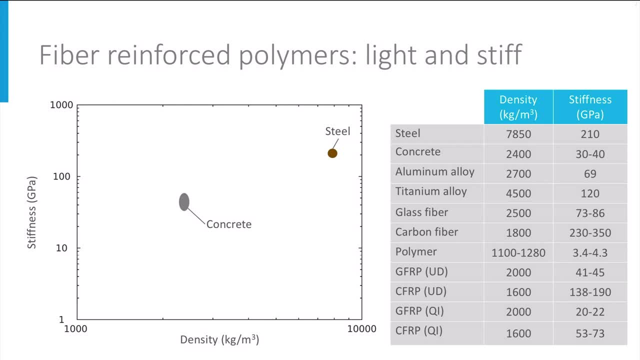 We start by placing steel and concrete. Steel has a density of almost 8000 kg per cubic meter and a stiffness of 210 GPa. The stiffness of concrete lies between 30 and 40 GPa at a density of 2400 kg per cubic. 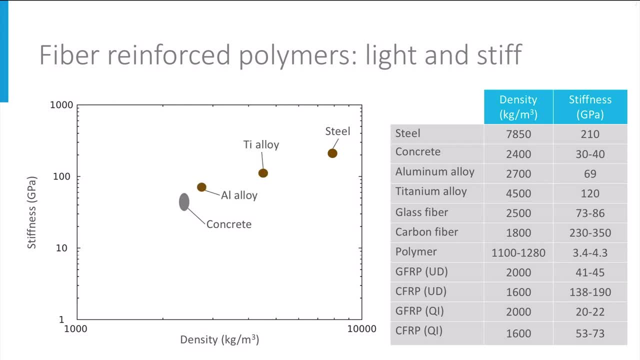 meter. Aluminum alloys are approximately 2 times more stiff than concrete. The density of aluminum alloys is approximately 2 times more stiff than concrete. The density of aluminum alloys is approximately 2 times more stiff than concrete. The density of aluminum alloys is approximately 2 times more stiff than concrete. 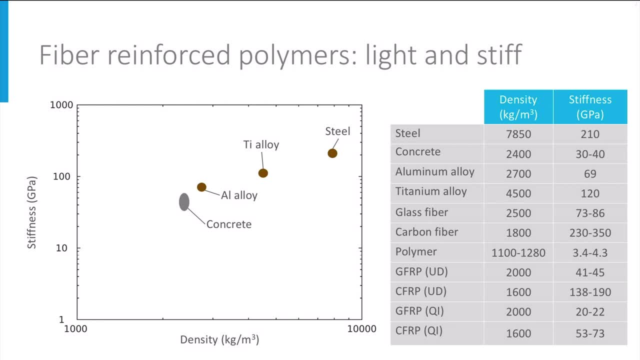 At almost the same density, while titanium lies somewhere in between aluminum and steel. Let's put some ingredients of FRP's in this chart. Glass fibers have a density that is comparable to concrete and aluminum and a stiffness that is somewhat higher. The Young's modulus of glass fibers lies around 70 to 80 GPa.